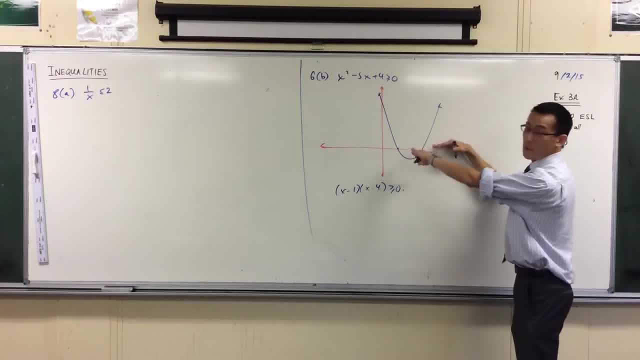 That's where I'm actually going to have solutions. What are the parts that correspond to above? Well, including the boundary, I'm here to the right- Should be on the line, sorry. And then I'm here to the left And of course, I know what these values are. okay. 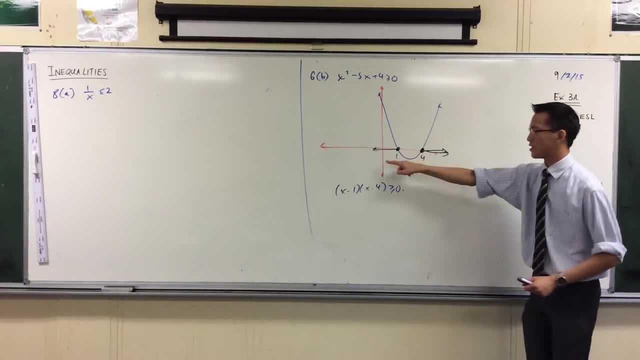 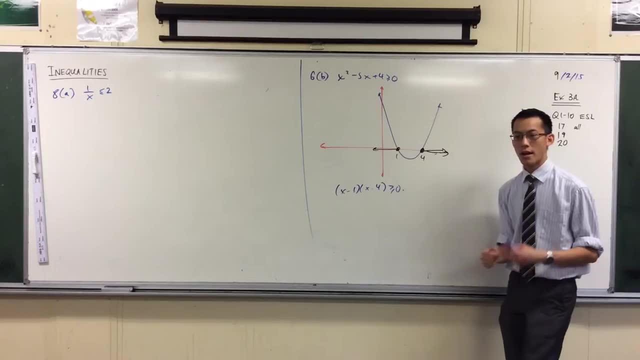 Now being that the solution to this inequality represents two completely separate regions Less than one, Less than or equal to one, Greater than or equal to four. It is worth writing this as two separate algebraic functions Like so: X is less than or equal to one. 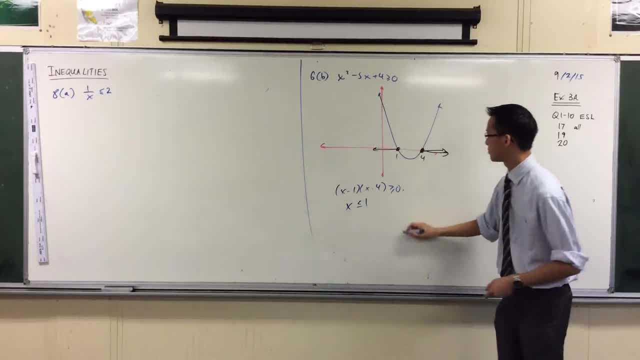 Or x is greater than or equal to four. Okay, Yes, Did you get it wrong? Instead of highlighting the parts like the four and the answer and the four and the one, did you highlight the part of the parabola? 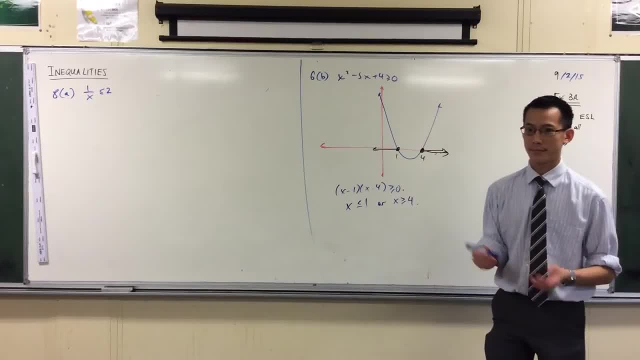 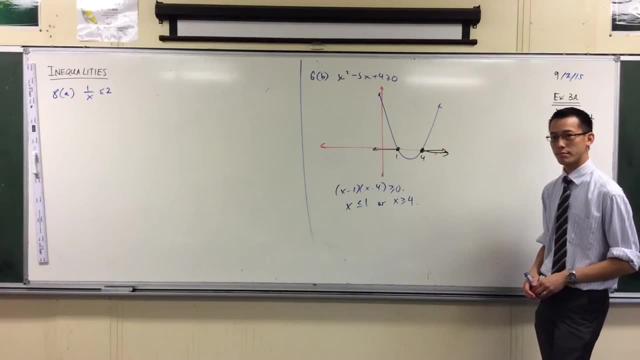 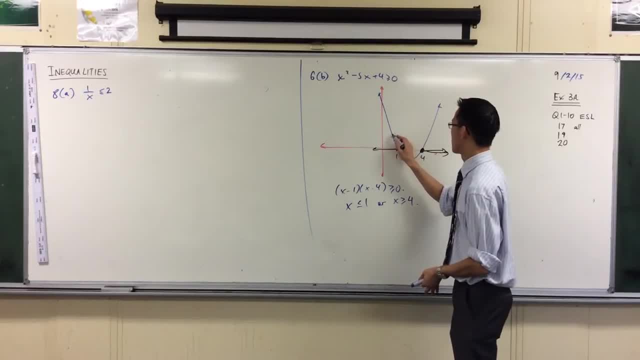 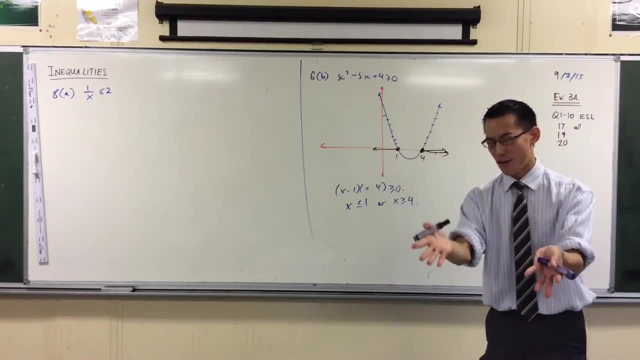 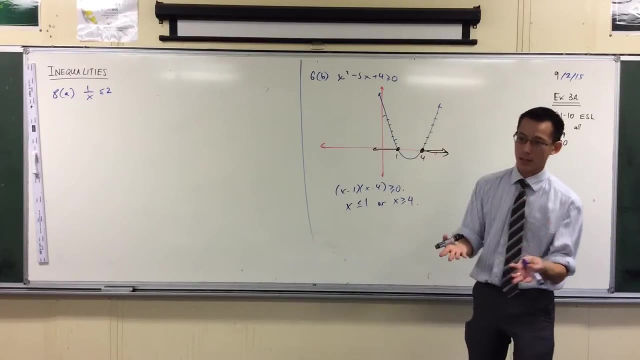 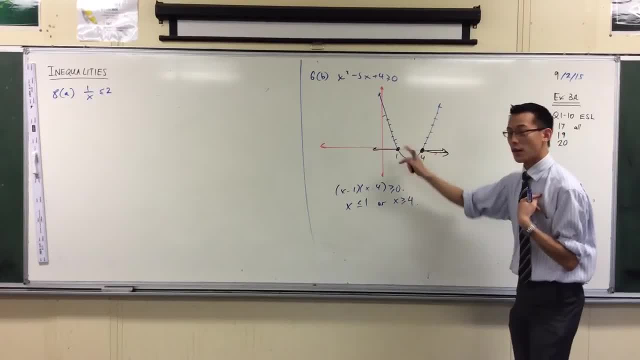 answer. So it's for me, really, This is for me. So if you did this, if you did these dots, that's fine. And then you wrote down this, okay, Because you would correctly represent the correct part. 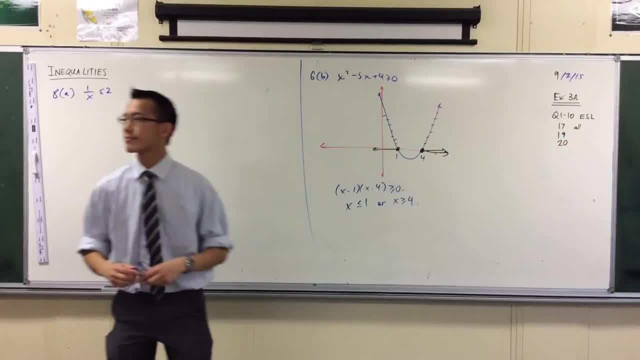 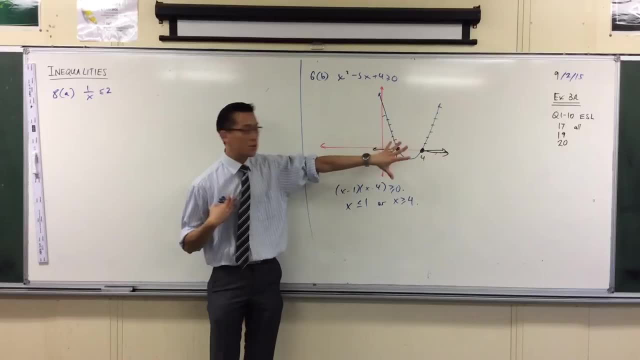 It makes more sense for me. Yeah, yeah, That's totally fine, I don't know. Yeah, it's fine. To be honest, I'm doing all of this extra stuff because I'm trying to illustrate my brain to you, right. 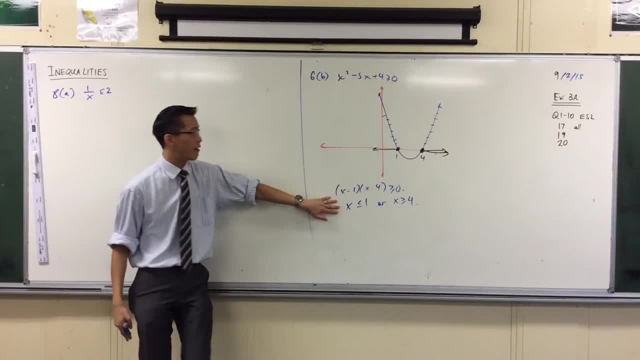 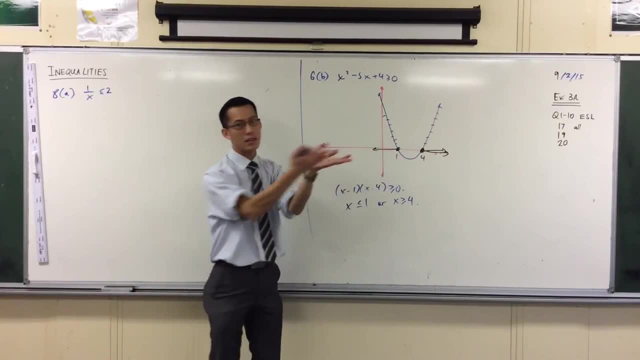 But if it was just me and my brain- and this is my end point, right? I don't need to do any of these markings, because I've seen this question so many times before and I'm familiar with the fact that what I'm looking for is the parts of the parabola above the axis and including the axis. 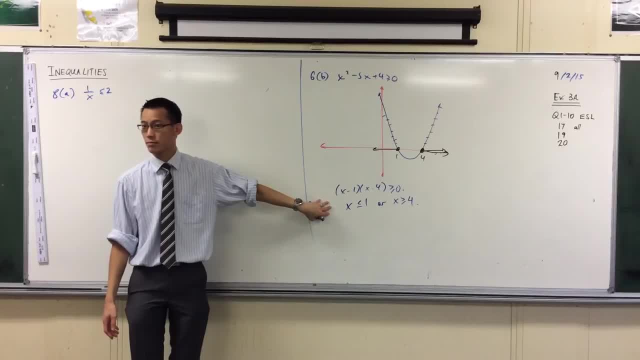 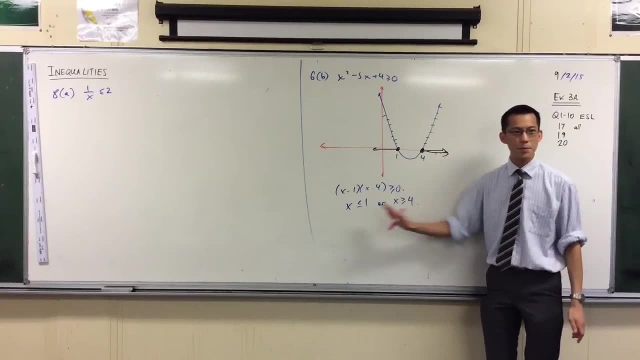 So you don't need to make any markings at all so long as you arrive at this conclusion. okay, Now it's worth saying that I'll do it in red. Some people insist on taking these values just to make sure I get this right, and writing them like this: